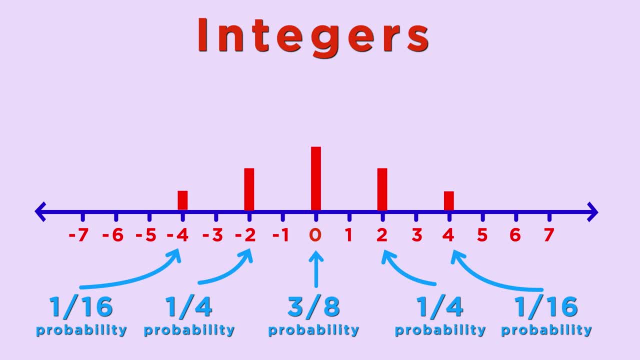 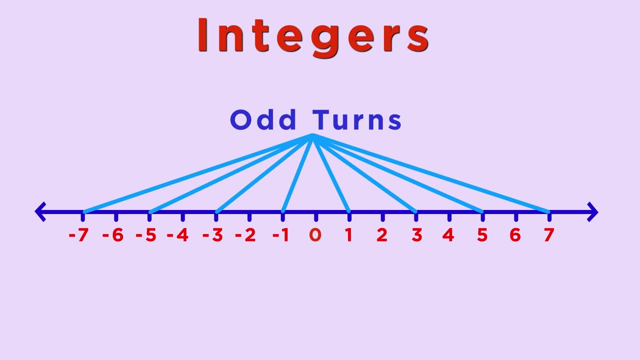 one sixteenth it's plus four. one quarter it's minus two. one quarter it's plus two, and three eighths it's zero. Here's a few observations. First on the odd turns. the random walk can only be on odd numbers and on the even turns. 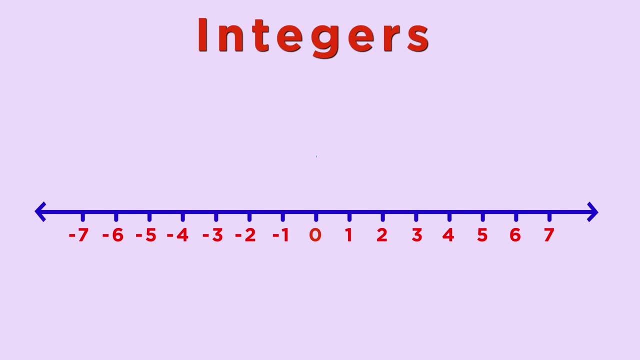 it can only be on even numbers. Second, it mostly hovers around the middle, the number zero. but the longer you flip the coin for, the more it can spread out. The probabilities of a random walk being in a specific location begin to form a bell curve. 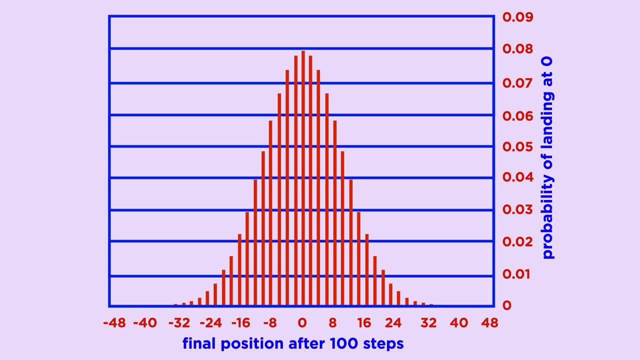 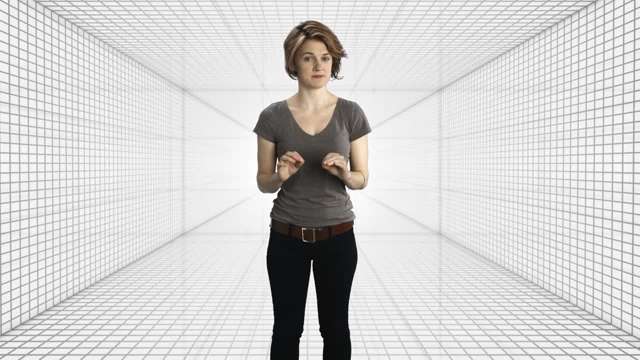 Notice that in the picture of the probability distribution after 100 coin flips, most of the time you'll be between plus 10 and minus 10.. Here's the more general version of that statement: After n coin flips, you'll usually be between minus square root of n and plus square root. 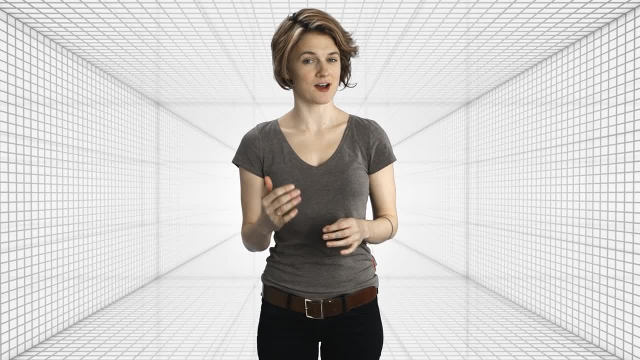 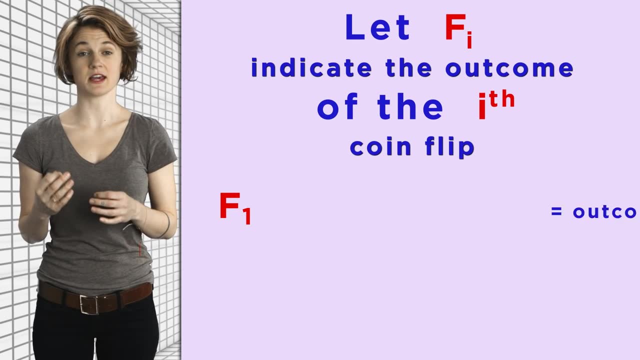 of n. Let's introduce some notation so that we can make this second observation more precise. Let fi indicate the outcome of the i-th coin flip. So f1 is the outcome of the first coin flip, f2 is the outcome of the second, and so on. 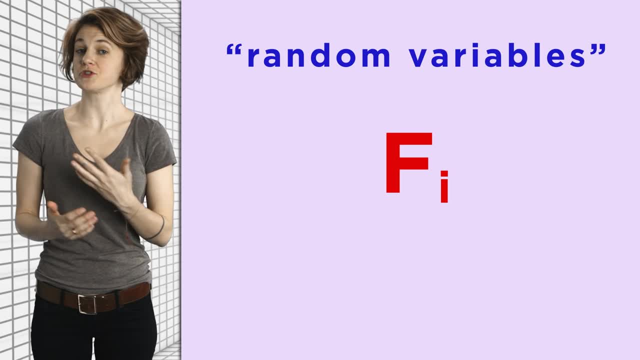 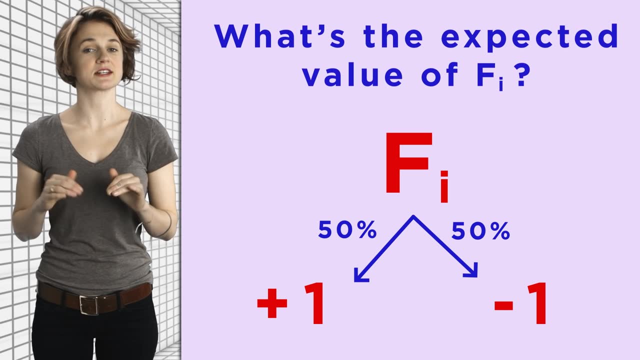 The fi are what's called random variables. The variables don't have a prescribed outcome. They have a 50% chance of being plus 1 and a 50% chance of being minus 1.. So what's the expected or average value of fi? 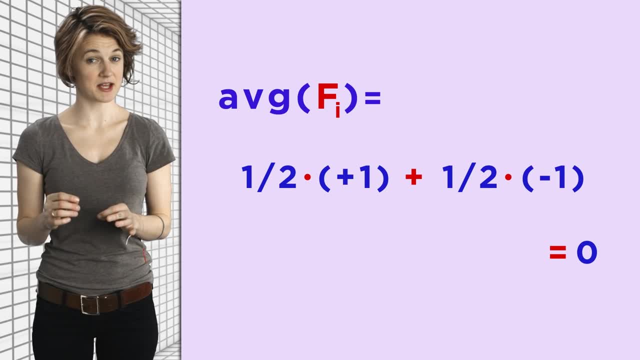 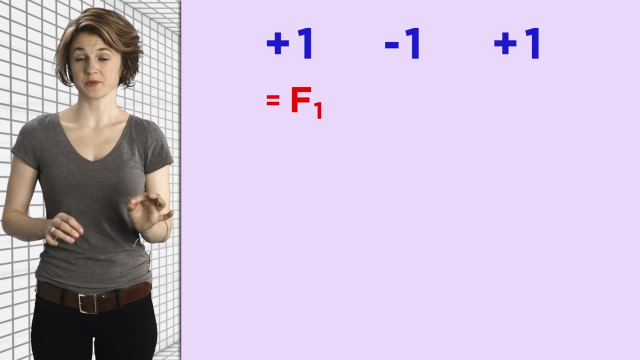 We calculate 1 half times plus 1, plus 1 half times minus 1.. So the expected value is zero. After we actually flip the coin, the fi have specific values. So if your first three flips are plus 1, minus 1, plus 1, then f1 equals plus 1, f2 equals 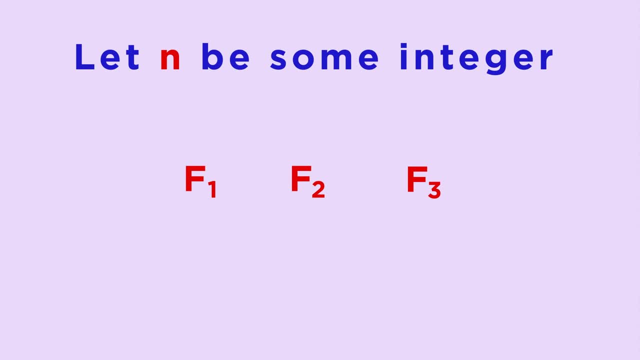 minus 1, and f3 equals plus 1.. Let n be some integer. If we add f1 plus f2 plus f3, all the way up to fn, together we get the location of the walk after n flips. Let's call that sn. 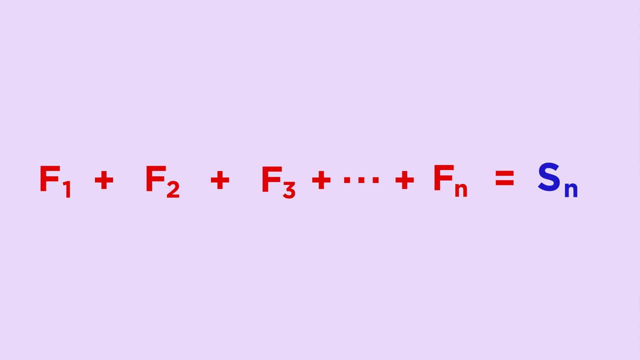 So sn, the sum of the coin flips, is also a random variable. It's actually the graphs from before that look like bell curves. So s1,, which is just f1, has a 1 half chance of being plus 1 and a 1 half chance of being. 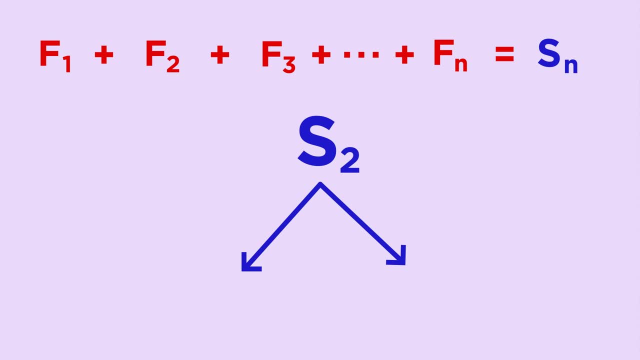 minus 1.. And s2, the location after two flips, or f1 plus f2, has a 1 quarter chance of being minus 2, a 1 quarter chance of being plus 2, and a 1 half chance of being zero. 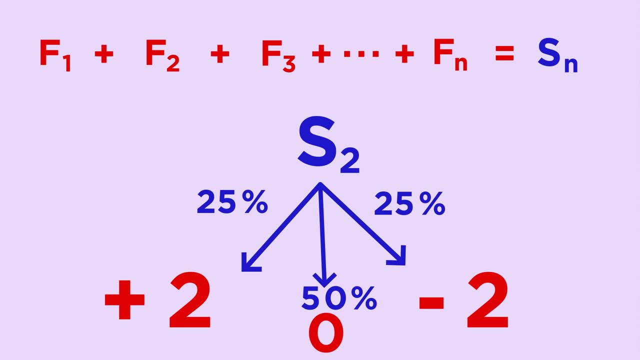 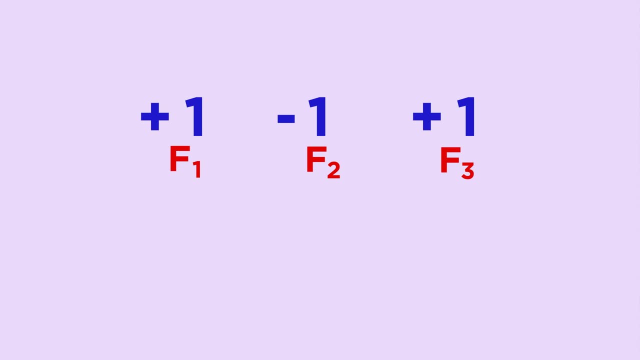 Again, these have specific values after you flip. So if your first three flips are plus 1, minus 1, plus 1,, then f1 equals plus 1, f2 equals minus 1, and f3 equals plus 1.. 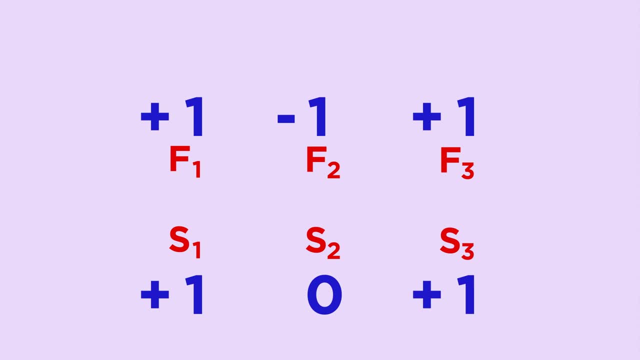 And s1 equals plus 1, s2 equals zero and s3 equals plus 1.. So what's the expected or average value of fi 1 half times plus 1, plus 1 half times minus 1.. Well, it's the sum of the expected value of the first n coin flips. 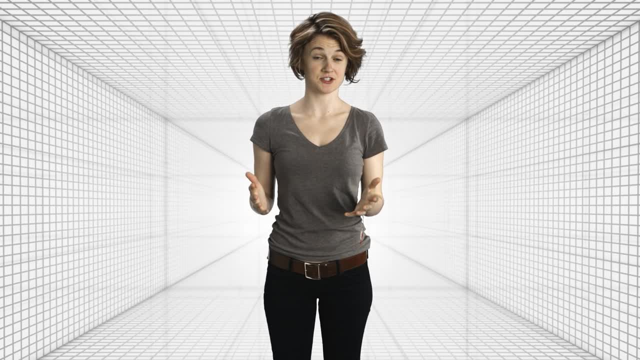 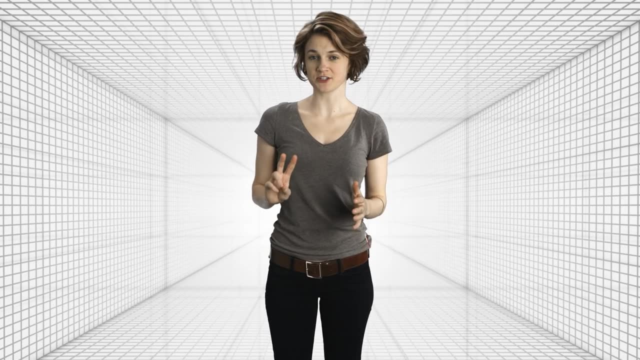 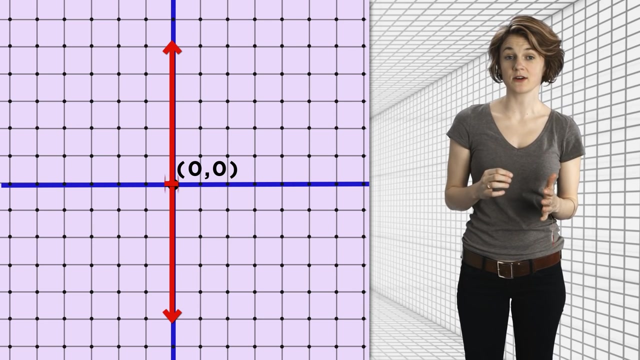 So it's zero. What we just looked at is a random walk on the integers, which is one-dimensional, But the whole thing works in any dimension. For example, on the two-dimensional integer lattice which looks like a grid, you start at the origin, the point 0,, 0,, and are equally likely to move up or down, or left or right. 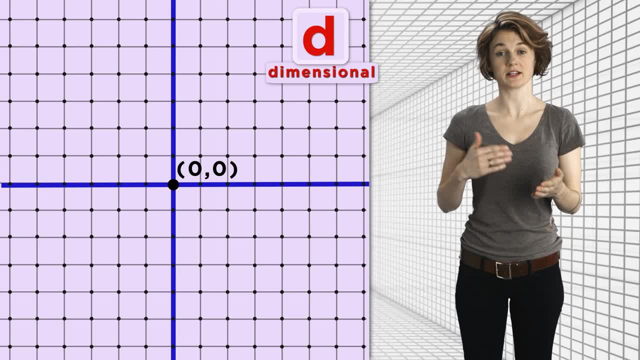 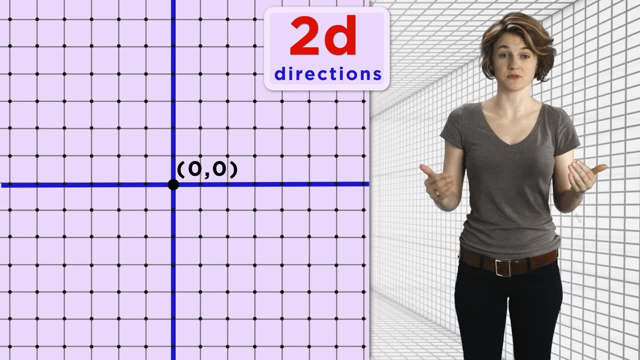 For an arbitrary number d. if you're randomly walking along a d-axis, you start at the origin d-dimensional integer lattice. there are 2 times d directions to move. Since you're equally likely to move in any direction, there's a 1 over 2 times d chance. 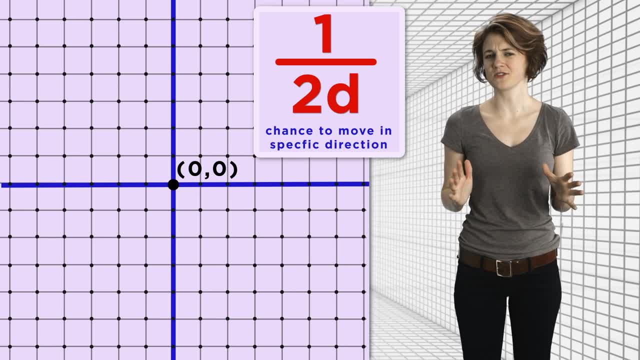 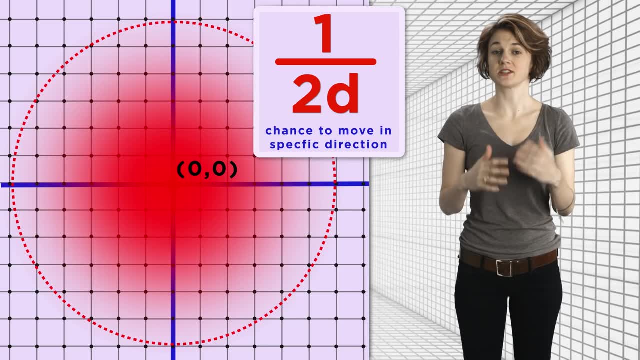 you'll move in a specific direction. Pretty much everything we've said so far is still true: You're still most likely to be at the origin. it's the expected value and after many steps, the distribution of the random walk will look like a bell curve, but in higher dimensions. 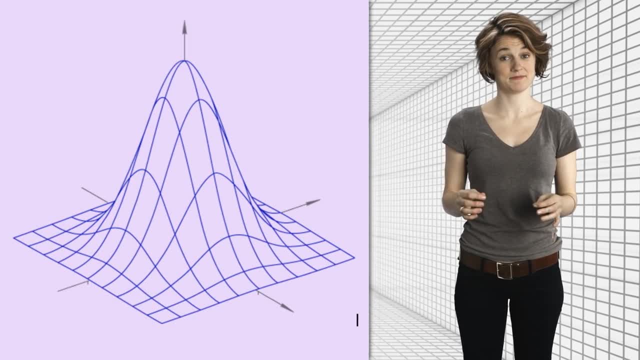 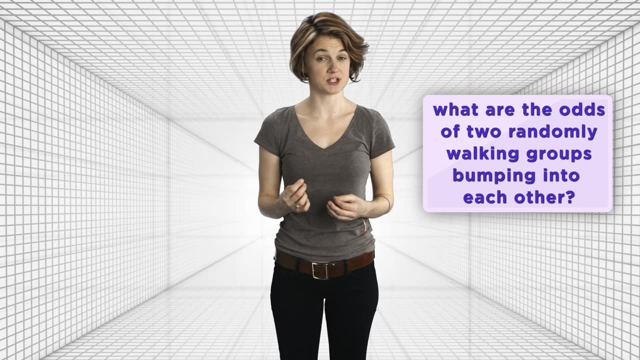 So for a two-dimensional lattice, the distribution actually looks like a bell. So back to Polya's question from the beginning: What are the odds that two independent random walks bump into each other? He quickly realized that in the case of a random walk on the integer lattice, this is: 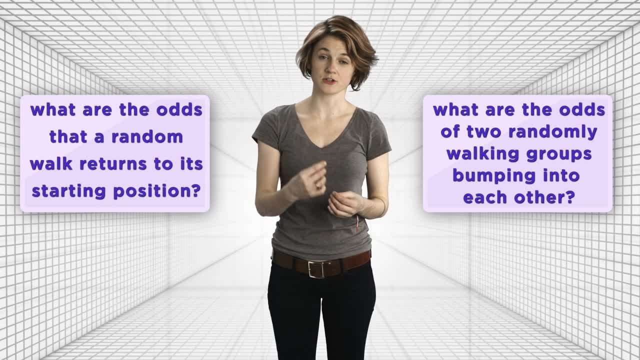 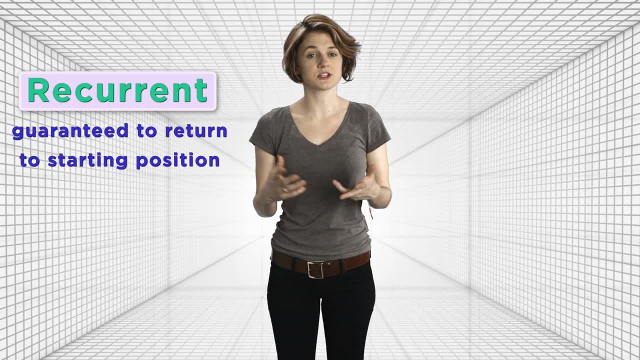 the same as asking what are the odds that a random walk returns to its starting position. Here's two definitions: Call a random walk recurrent if it's guaranteed to return to its starting position. Call a random walk transient if there's a positive probability that it never returns. 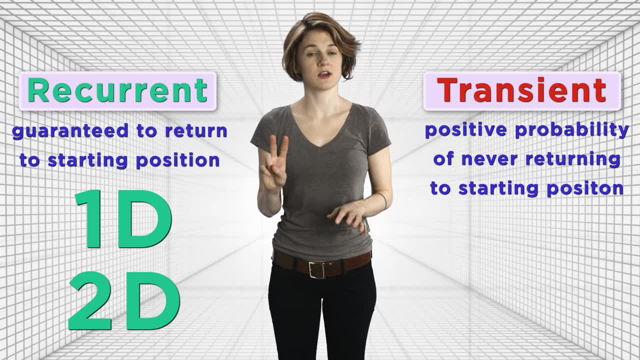 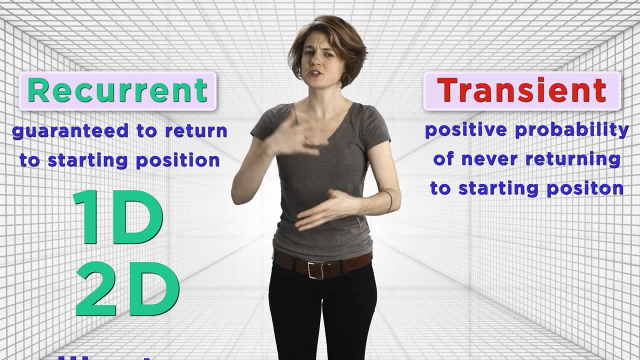 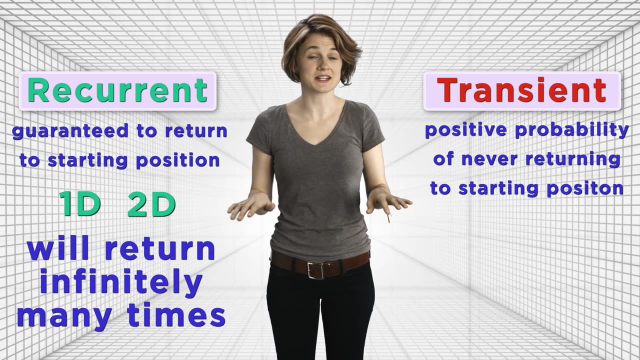 to its starting position In one and two dimensions. a random walk is recurrent. There's a 100% chance it returns to its starting spot. In fact it'll return there infinitely many times. So that answers Polya's question. They're walking along the two-dimensional ground and guaranteed to keep bumping into. 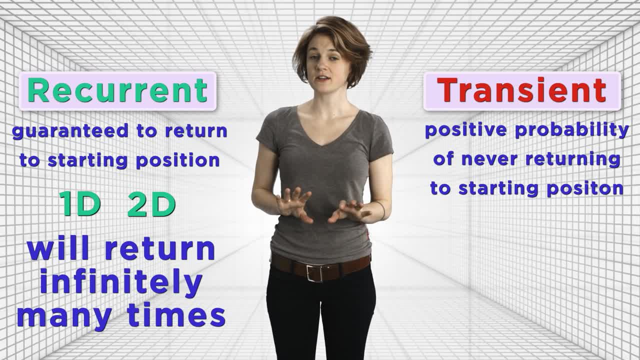 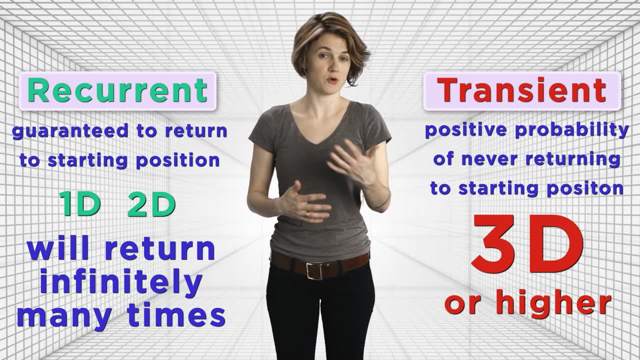 each other over and over again. But a random walk on the integer lattice in dimensions 3 and higher is transient In 3 or 4 or 5, it's transient In 1 or 100 dimensions. there's a chance that the random walk will escape and never. 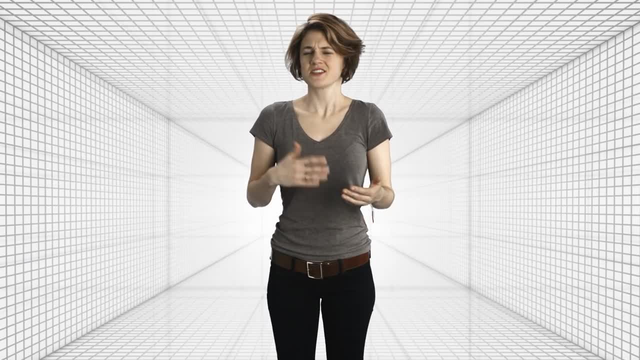 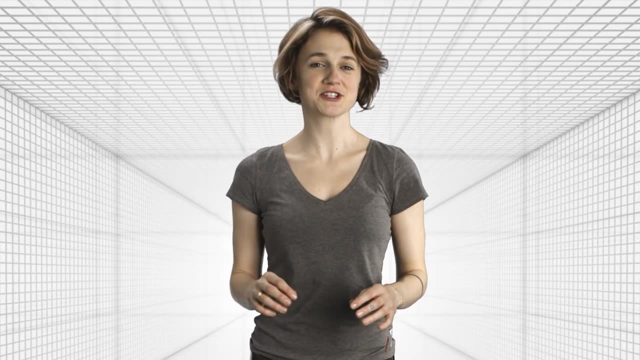 return to its starting spot. Intuitively, this kind of makes sense. In higher dimensions there's more space or options for where a random walk can wiggle off to. A favorite joke among mathematicians is: a drunk man will eventually find his way home. 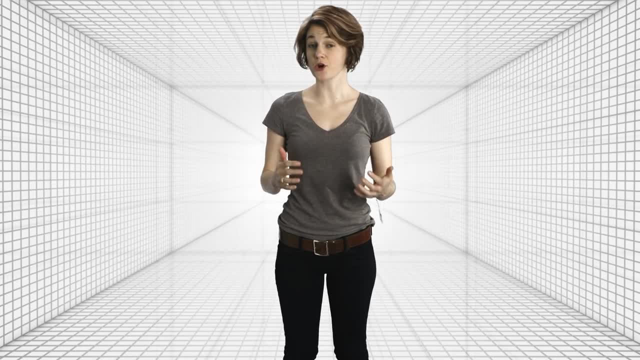 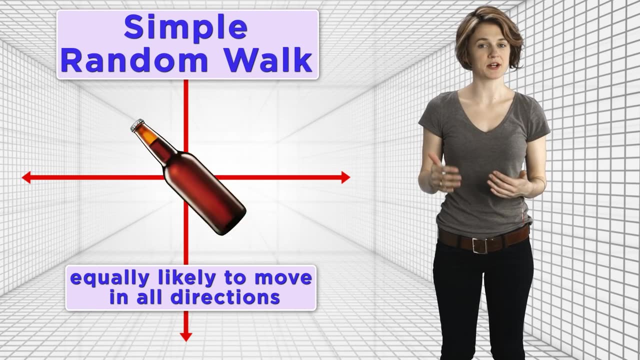 but a drunk bird may get lost forever. The drunk man has no preferential direction. He's equally likely to move in all directions. We call that a simple random walk, But in general a random walk can have a bias or a preferential direction. 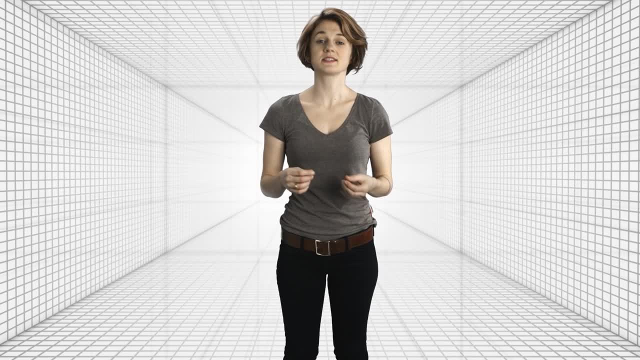 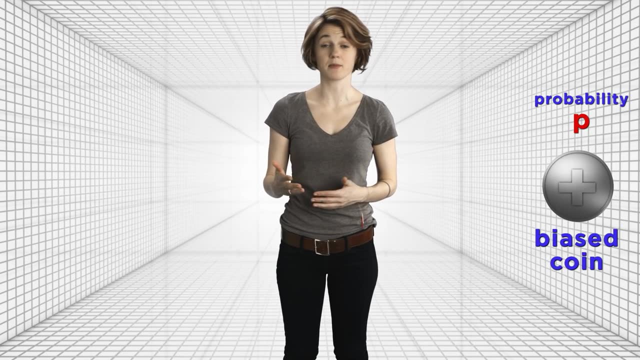 Let's look at this in one dimension. Now, instead of flipping a fair coin, you're flipping a biased coin. It has probability p of landing on plus and probability 1 minus p of landing on minus, where p is some number between 0 and 1.. 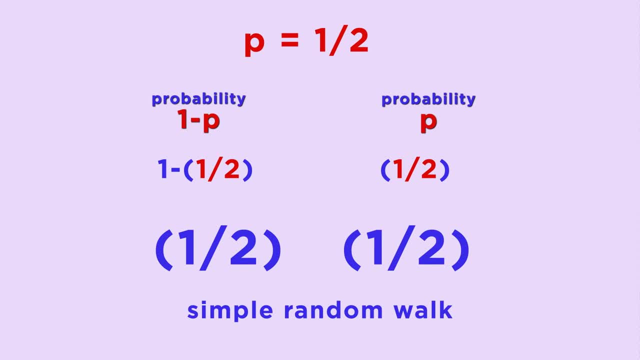 So if p equals 1 half, we have a simple random walk we were just looking at. But if p equals 1 quarter, it has probability 1 quarter of moving right and probability 3 quarters of moving left. So it's three times more likely to move left than right. 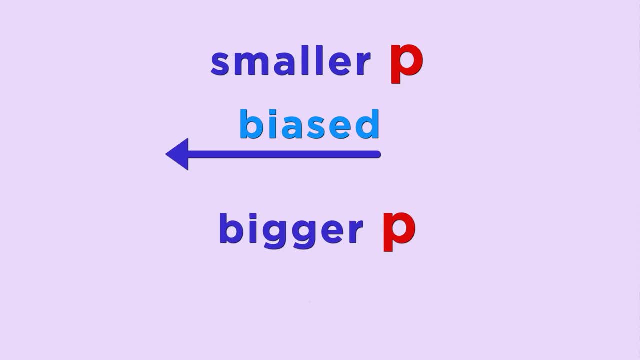 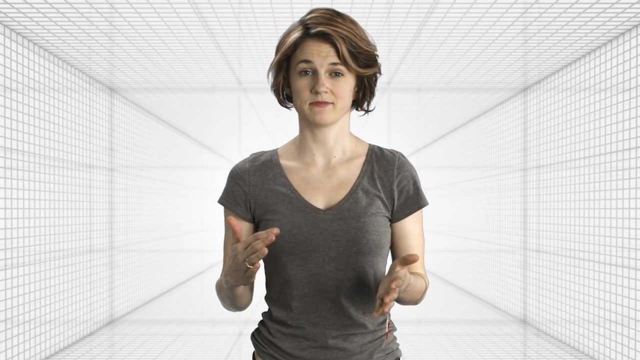 The smaller p is, the more it's biased to the left. The bigger p is, the more it's biased to the right. Before we expected our random walk to hover near 0. But now it should be moving. Let's look at a similar computation as before to find out the expected value of one coin. 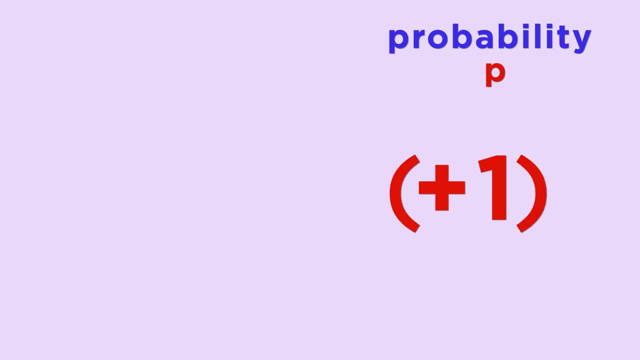 flip. With probability p, the coin flip is plus 1.. And with probability 1 minus p, the coin flip is minus 1.. So the average value of the coin flips will be 2p minus 1.. Where will it be after n steps? 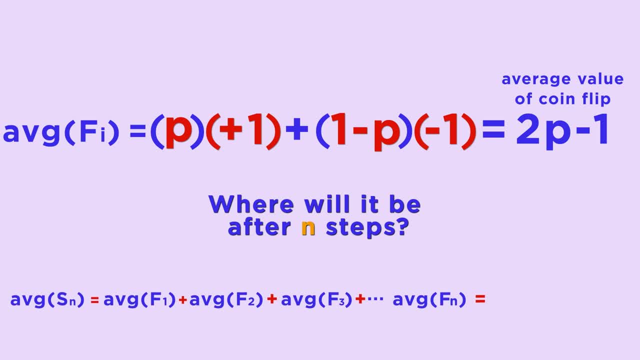 Let's compute the expected value Again. it's the sum of the expected values of the n flips, So it's n times 2p minus 1.. For the sake of example, let's assume p equals 3 quarters. That means there's a third. 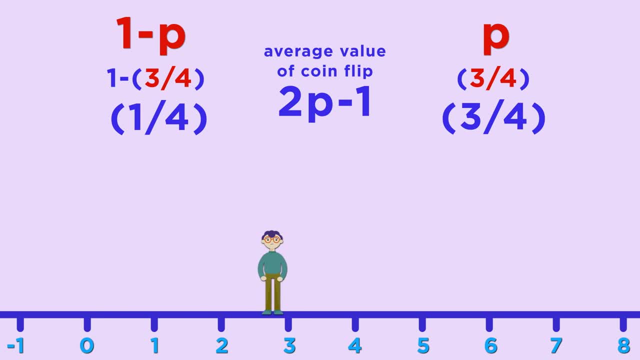 There's a 3 quarter chance of moving right and a 1 quarter chance of moving left. So 2p minus 1 equals 1 half. So after 10 moves you'd expect to be at plus 5.. And after 100 moves you'd expect to be at plus 50.. 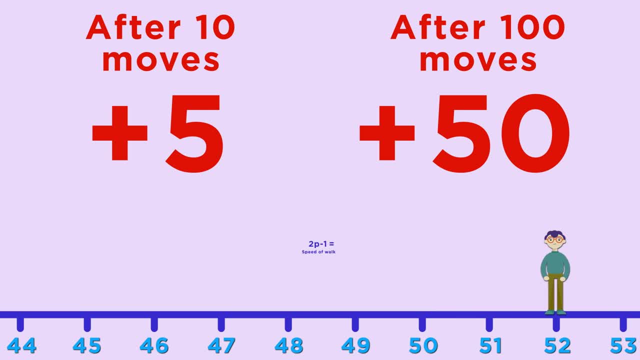 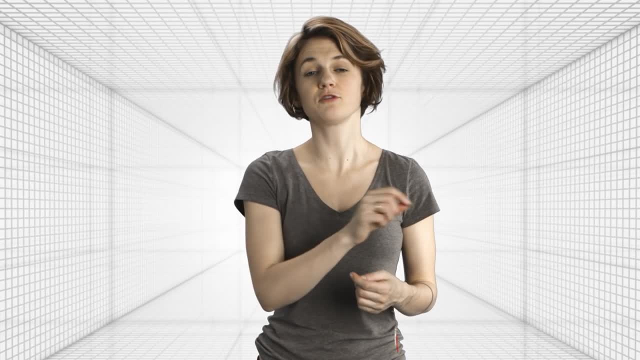 You're moving to the right with speed 1 half. So 2p minus 1 is like the speed of the walk. But the random walk isn't going to move at exactly that speed. It'll fluctuate around that average, Just like the simple random walk fluctuated around 0.. 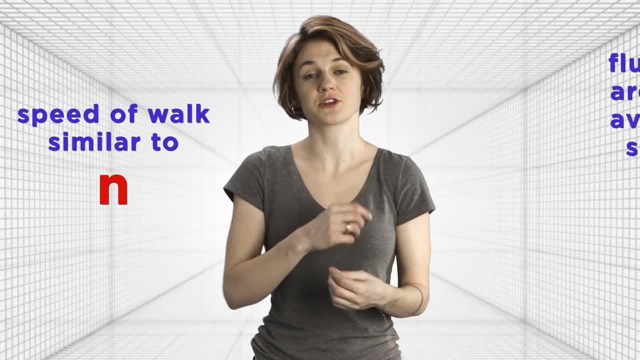 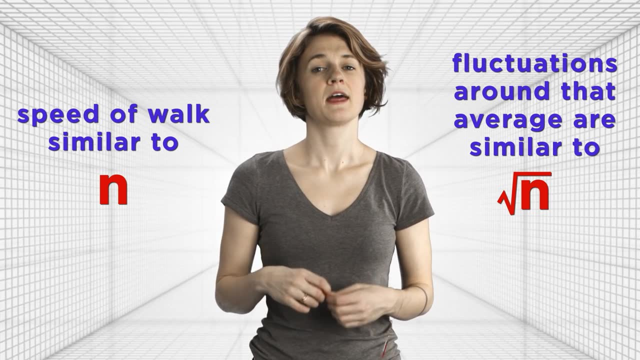 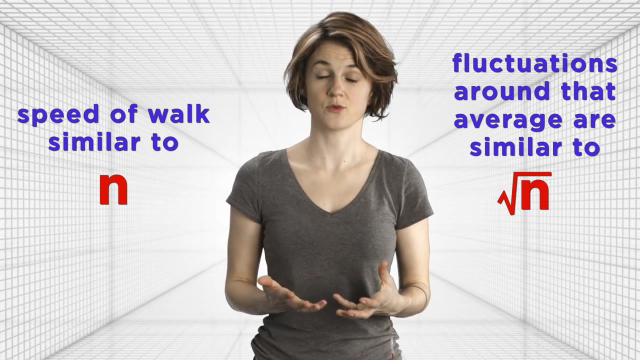 While the speed of the walk is similar to n, the fluctuations around that average are similar to the square root of n. So there's really two speeds happening here: The average speed at which it's moving, which is like n, and the speed at which it's fluctuating around that average. 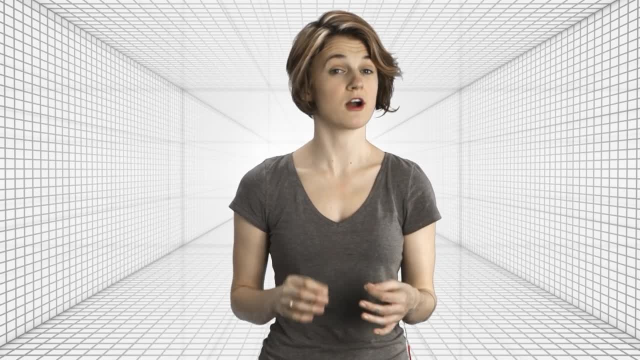 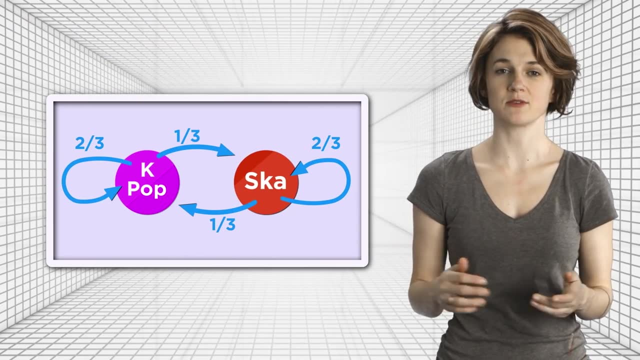 which is like the square root of n. I want to point out for folks who saw our episode on Markov chains that a random walk is an example of a Markov chain. Remember that a Markov chain was a set of states with arrows connecting them. that told us. 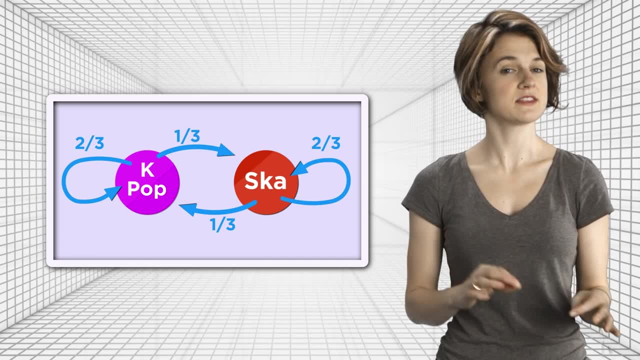 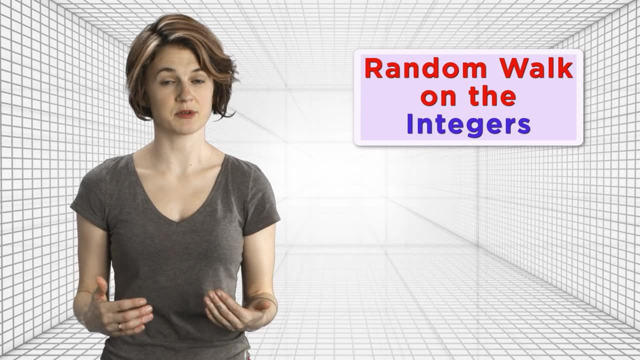 how likely you are to jump from one state to another. In that episode we only looked at Markov chains with finitely many states, But a random walk on the integers is an example of a Markov chain with infinitely many states. Each of the infinitely many integers is a state. 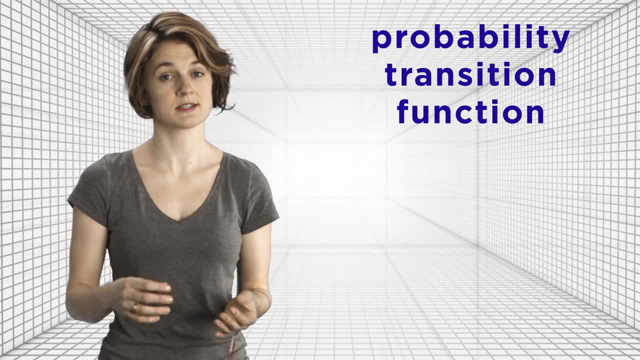 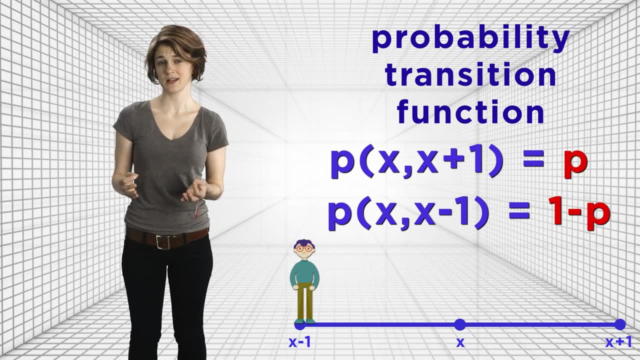 And the probability transition functions are given by the equations: probability of jumping from x to x plus 1 equals p and the probability of jumping from x to x minus 1 equals 1 minus p. Random walks are everywhere, They're not just on the integer lattice. 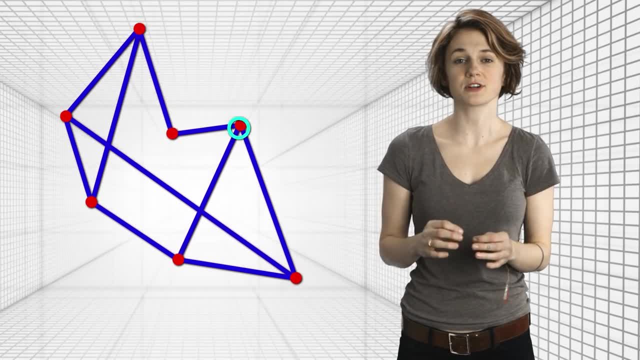 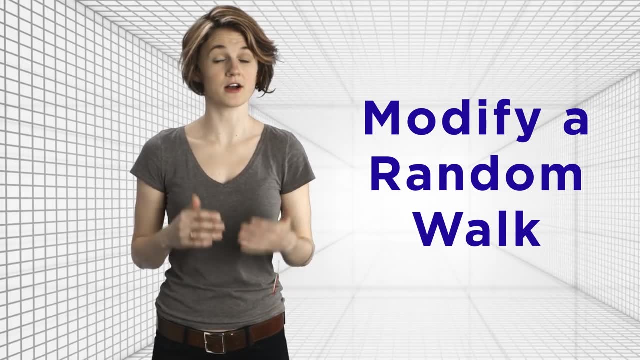 You can randomly walk through a graph like this. A computer can randomly walk through websites, which is basically what Google's search algorithm is doing. You can modify a random walk on the integers by requiring that it stop if it hits plus 10 or minus 10,. 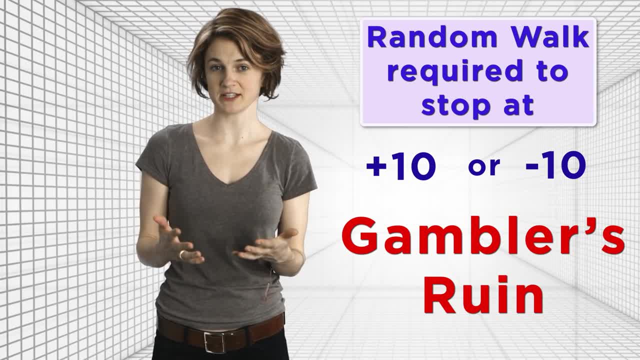 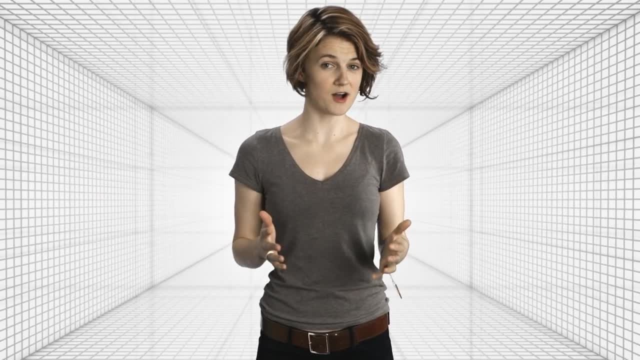 what's known as gambler's ruin, a model of a simple gambling game. You can also use random walks to model the stock market. There's an endless number of interesting random walks. What's your favorite? Let us know in the comments. 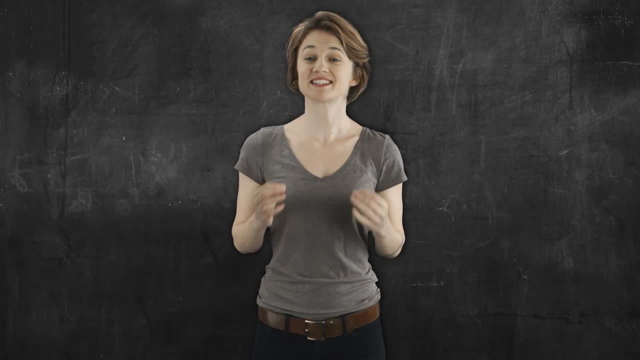 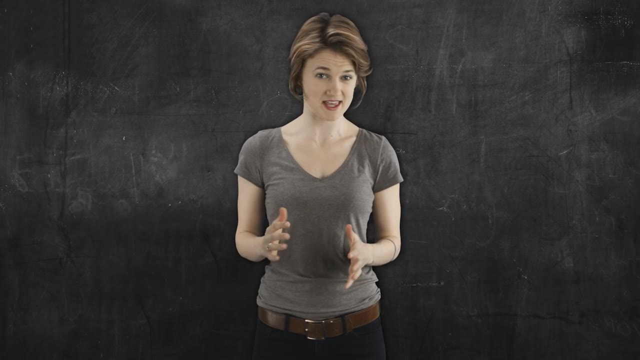 See you next week on Infinite Series. Hey, all, It's time for the annual PBS Digital Studios survey. How did PBS react to the nearly 40,000 responses they got last year? By creating this show. You all asked for a math show and you got it. 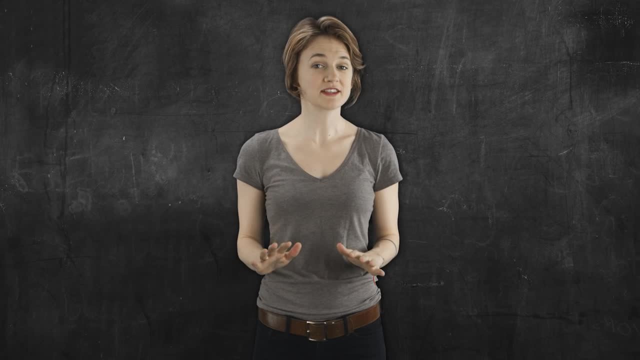 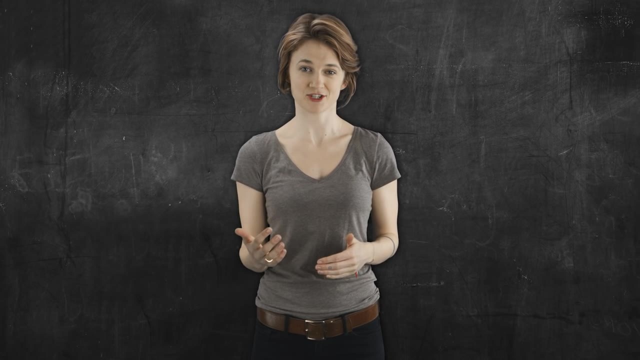 So what do you want to see on YouTube in this upcoming year? There's a link in the description to the survey. It should only take 10 minutes to fill out and 25 randomly selected participants get PBS t-shirts. We're excited to hear what you're thinking. 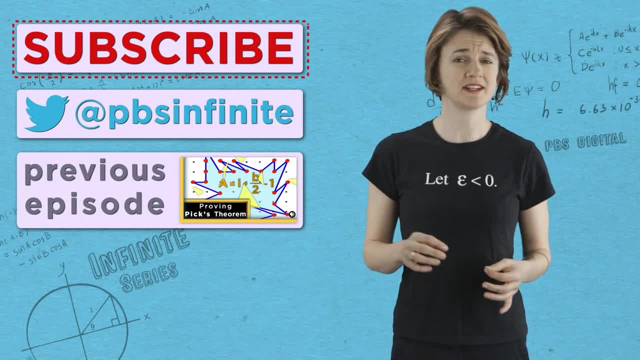 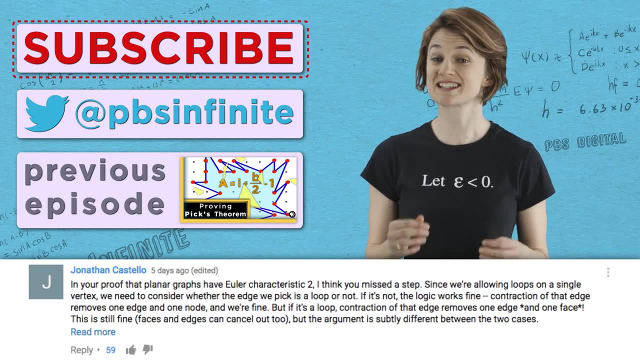 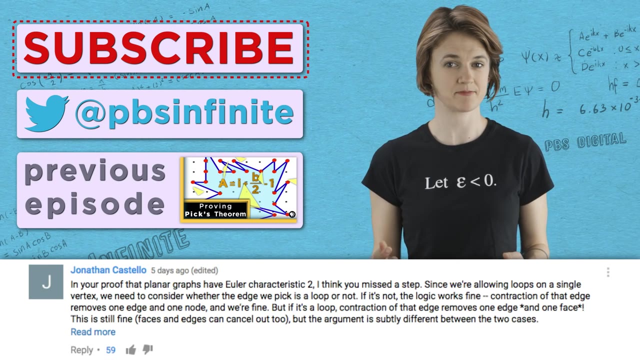 Let's talk about your responses to Pick's theorem, the formula for finding the area of polygons with vertices on the integer lattice. First, Jonathan Castello has an excellent correction. He says in your proof that planar graphs have Euler characteristic 2, I think you missed a step. Since we're allowing loops on a graph. I think you missed a step, Since we're allowing loops on a graph. I think you missed a step, Since we're allowing loops on a graph. I think you missed a step, Since we're allowing loops on a single vertex. 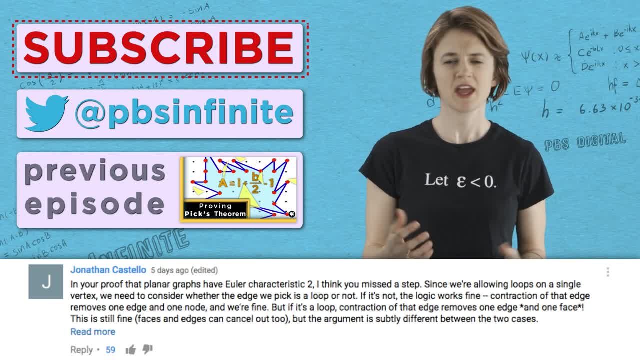 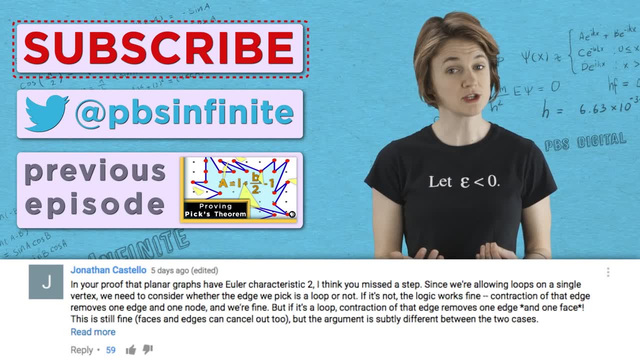 we need to consider whether the edge we pick is a loop or not. If it's not, the logic works fine. Contraction of that edge removes one edge and one node and we're fine. But if it's a loop, contraction of that edge. 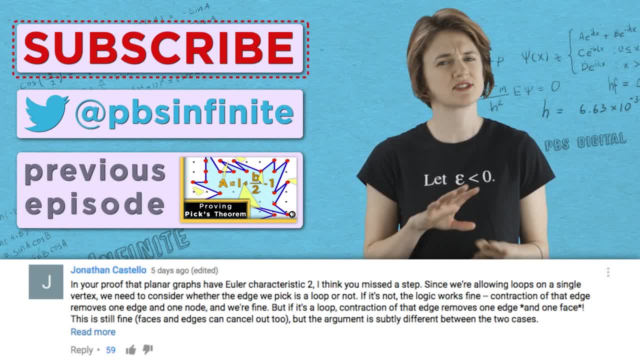 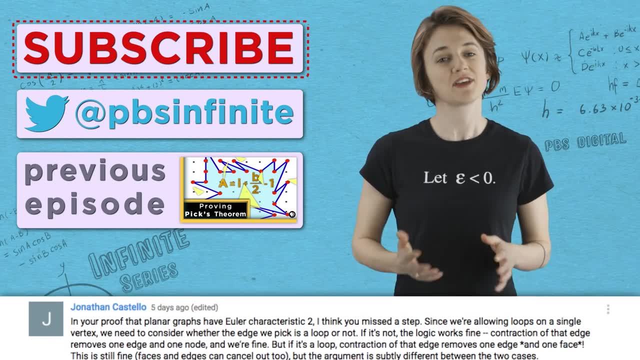 removes one edge and one face, This is still fine. Faces and edges can cancel out too, But the argument is subtly different between the two cases. Thanks for pointing that out. Jonathan Petros Adamopoulos responded that this method is actually not the simplest. 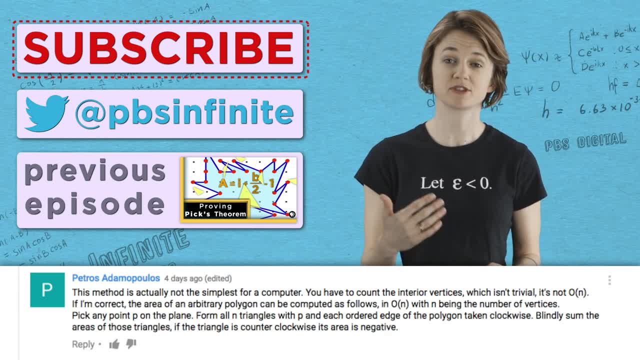 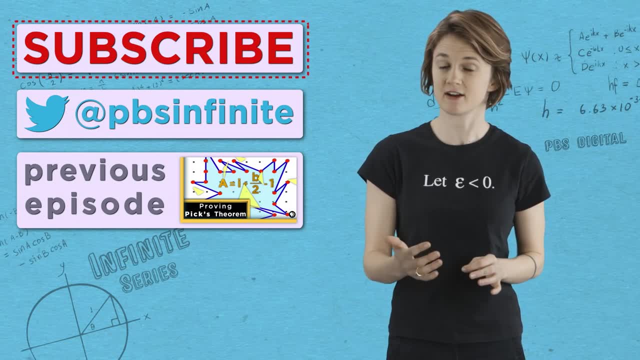 It's the simplest for a computer, and then suggested a method for a computer to find the area of a polygon. This made me curious. Does anyone know other methods for a computer to find the area of a polygon? What about an arbitrary shape? 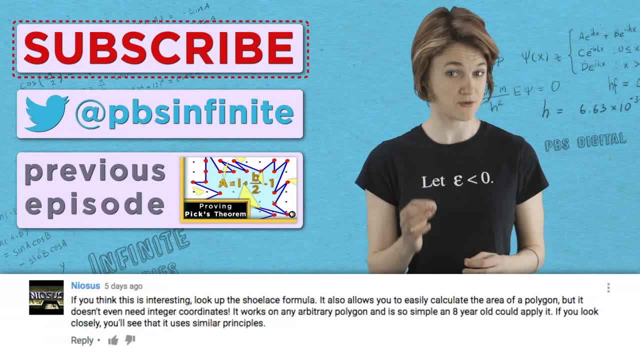 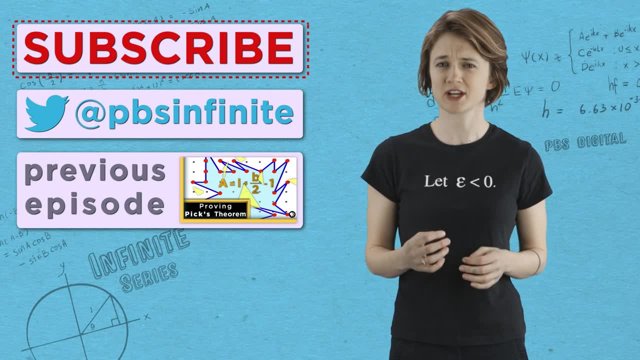 Finally, Gnosis drew our attention to the shoelace formula, which I'd never heard of before. It also finds the area of a polygon in a neat way that multiplies the vertex coordinates in a weird crisscross pattern. hence the name shoelace formula. 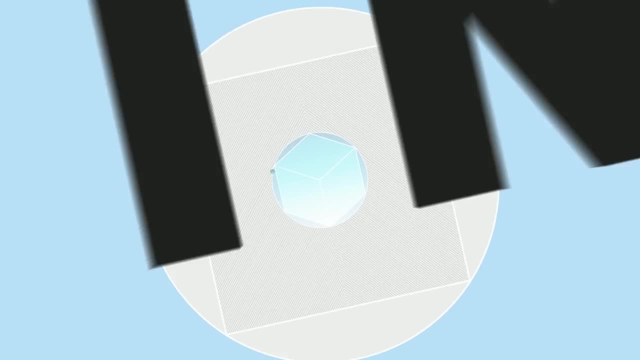 Go check it out. See you next time.